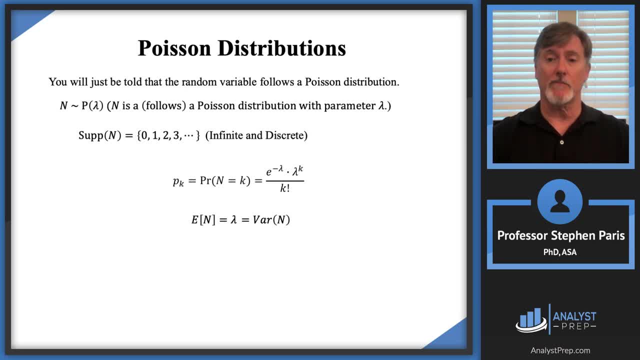 the expected value and the variance are equal to each other. They're both equal to that parameter, lambda. For that reason sometimes you might be told that this- you know it might be the problem- might say you have a Poisson distribution with a mean of lambda or 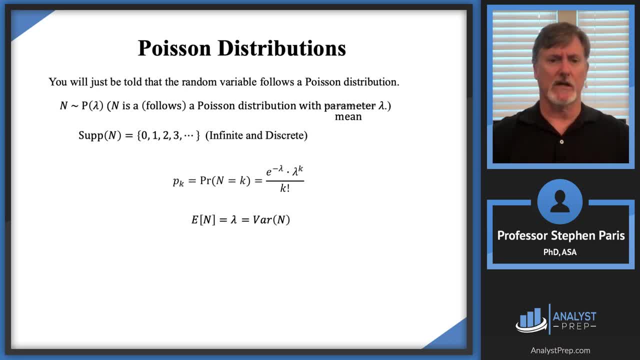 in a very rare instance, maybe it says a Poisson distribution with a, with a variance of lambda. Those they're all equal: The mean, the variance, the parameter. you'll probably most likely see just parameter lambda, But they're, they're all equal: The mean, the variance and the parameter. Okay, Let's look. 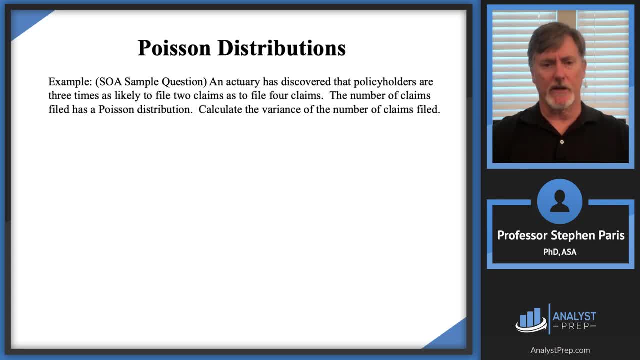 at an example. This comes from an SOA sample question for exam P. An actuary has discovered that policyholders are three times as likely to file two claims as to file four claims. The number of claims filed has a Poisson distribution. There you're just told that it has a Poisson distribution. 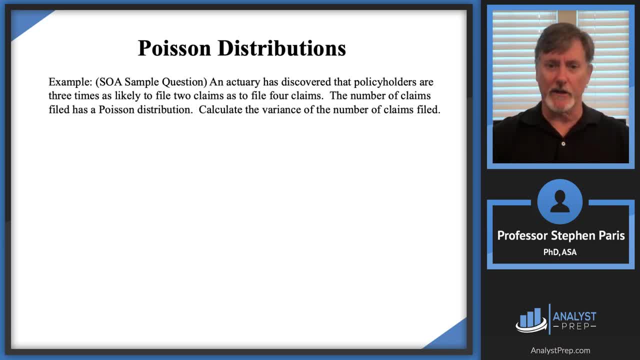 And we're asked to calculate the variance of the number of claims filed. So our solution- cap in is- is following a Poisson distribution, with this parameter, lambda, We seek the value of the variance of of of cap in. Well, that's just lambda, It is just a, a, a, a another way. 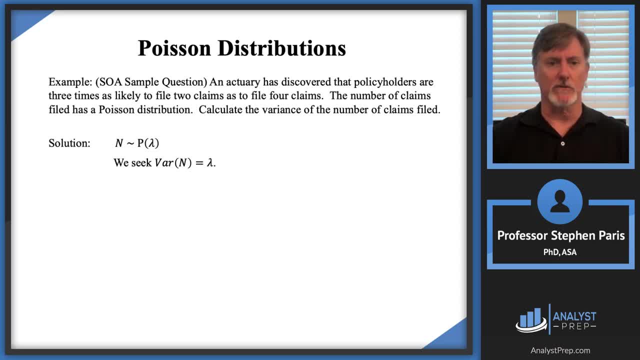 of saying what's? what's the parameter equal to, What's lambda equal to? So let's use the information that's given to us, Namely that policyholders are three times as likely to file two claims as to file four claims. So the probability of filing, uh, two claims is 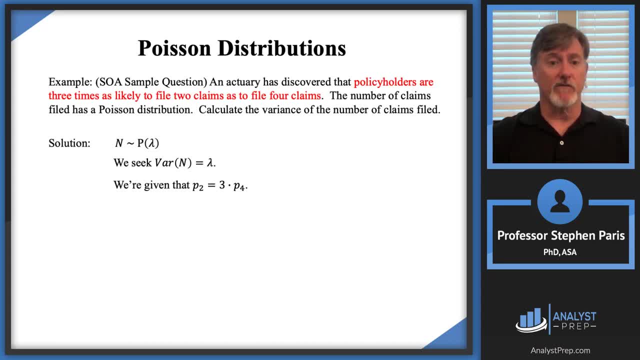 is is three times. whatever the probability is of file file filing four claims Uh. so the policyholders are three times as likely, more likely, that has a higher probability of uh of calculating uh of uh filing two claims. So the uh P sub two needs to. 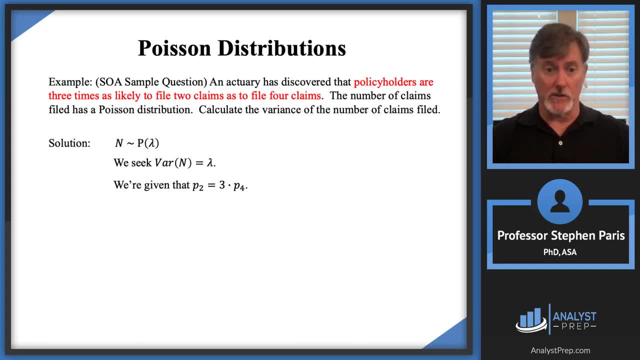 be a bigger value than P sub four. And not only is it bigger, we're told it's three times bigger than the uh the P sub four value. At this point, recall the formula for P sub K: generally It's E to the minus lambda. 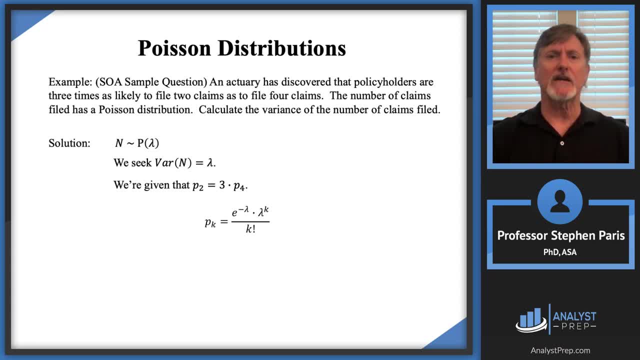 Lambda to the K divided by K factorial. So P sub two. I'm plugging in a two for K. P sub four. I'm plugging in a four for K. I get this, this equation, The E to the minus lambdas. 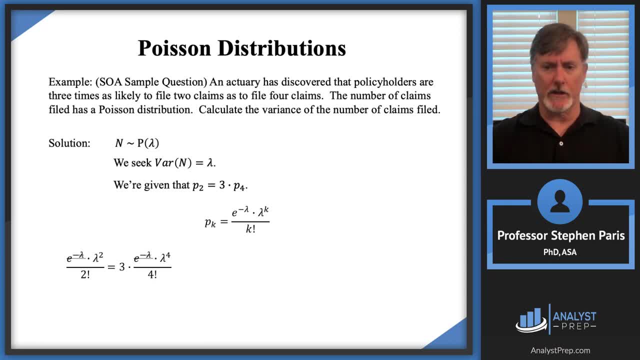 are gonna, are gonna, uh, uh, cancel off, And so, uh, you know, I, I'll get, I'll get this equation that I have shown, and just doing some arithmetic on the right hand side: Three, three and then divide by twenty-four, That's like divide. you know, just one eighth Um. 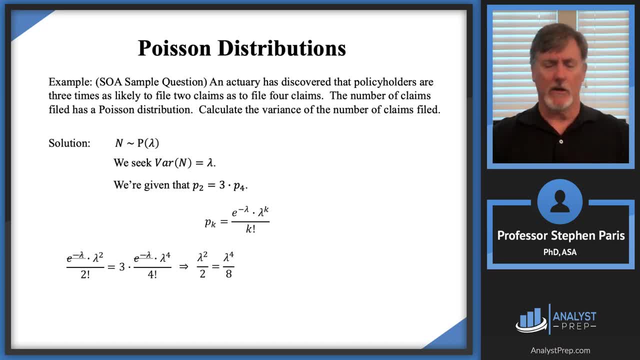 you cross, multiply or do some cancellations? Uh, whatever probability you have, uh, whatever process you're gonna go through, reduce this equation. Uh, you know, you cross, multiply and then, and then divide out by lambda squared And you'll see that lambda squared would be. 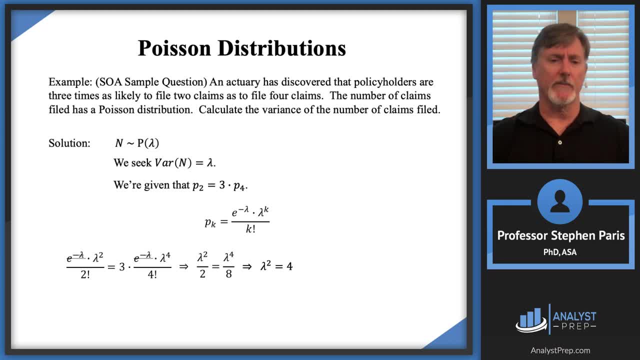 four, And generally, when lambda squared is four, your solutions are lambda would be plus or minus two, But your parameter's never gonna be negative. uh, it it for? for this distribution, The parameter is the variance. And so, uh, the variance is never negative, The parameter. 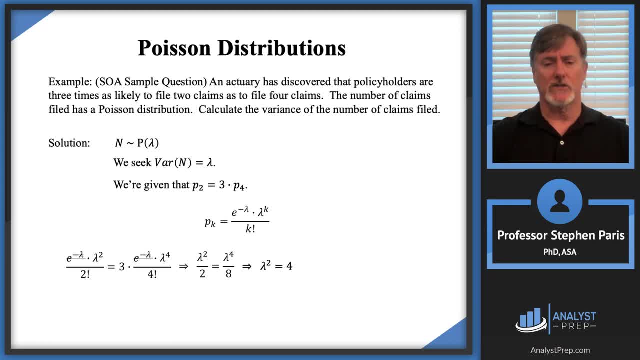 will never be negative, uh for Poisson distribution, And so um, uh, ignore the extremes, And so we get a simultaneous solution of negative two And we get that lambda equals two. So my answer here is that the variance of cap N is is two, The uh, the uh uh in the 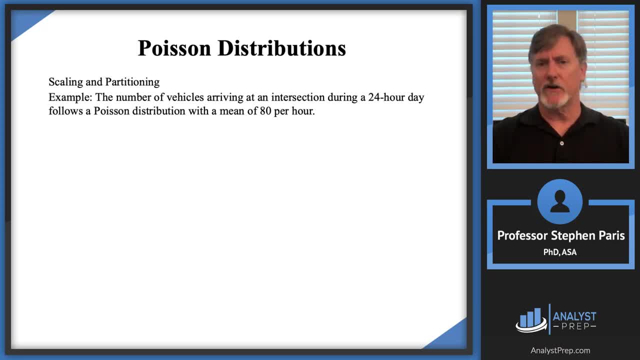 next slide here: uh, the uh Poisson distribution has some very nice properties And and uh. a couple of them are called scaling and and partitioning uh properties, And so let's talk about uh. for the rest of the video, I want to talk about scaling properties and. 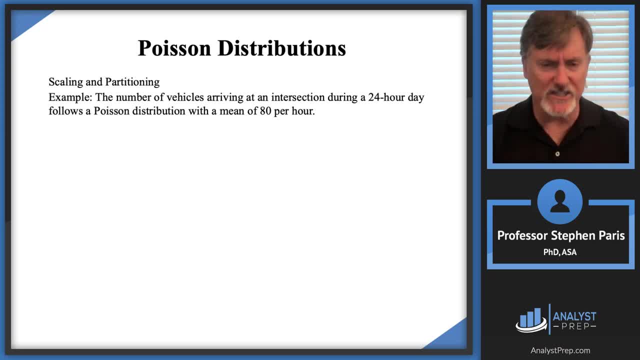 and partitioning properties. When, when we talk about scaling, what we're talking about is scaling the uh, what's called the exposure unit. So in this example, I have vehicles arriving at an intersection during a uh, a 24-hour 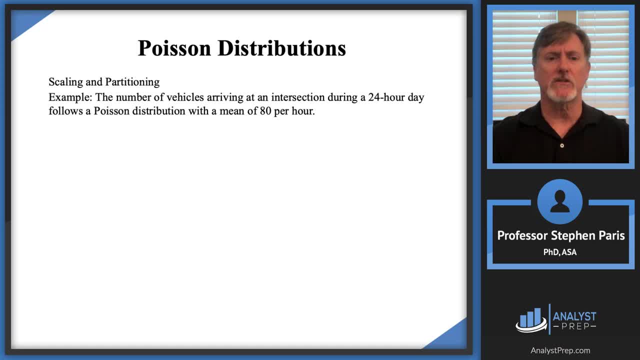 day: Uh, vehicles arriving at an intersection follows a Poisson distribution with a mean of 80 per hour. So whenever you're counting, uh, and, and that's what the Poisson distribution is, a counting distribution. It's what's called a frequency distribution. We're counting. 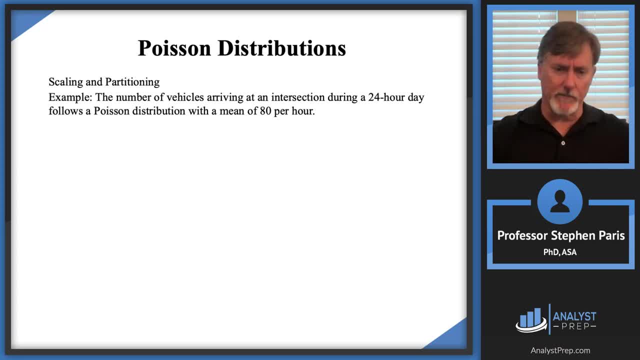 uh, things, And whenever you're counting, you're counting per something, in this case per hour, And that per something. when you're counting per something, the something is called the exposure unit. So the- in this case the exposure unit is in- is an hour. However, we might ask the. 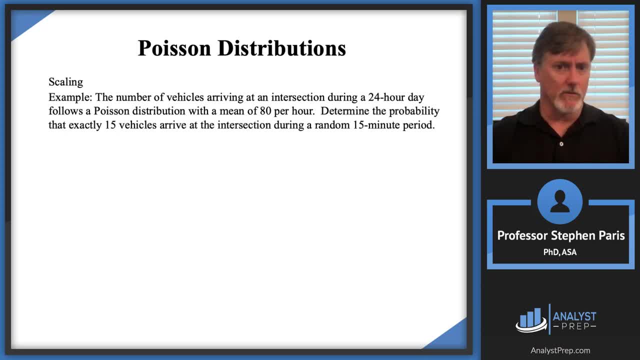 problem. Let's, let's, tweak the probability here. Or or right, uh, uh, ask for the probability. What's the probability that exactly 15 vehicles arrive at the intersection during a random 15-minute period? So I, I'm going from an hour to a 15 minute period. I'm going to scale. 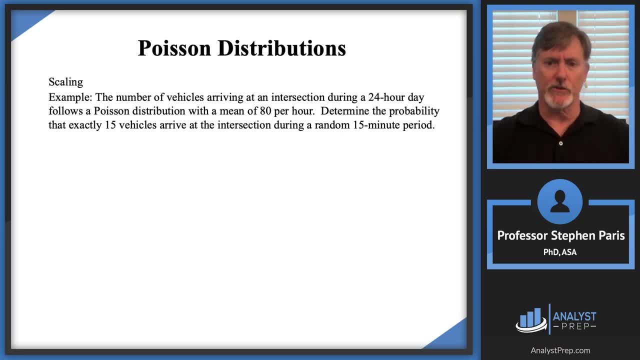 the. what I'm doing here is- I'm calling it- scaling the, the exposure unit, to a 15 minute period. So let me start, though, with the hour exposure unit. Cap in be the random variable representing the number of vehicles arriving at intersection per hour. 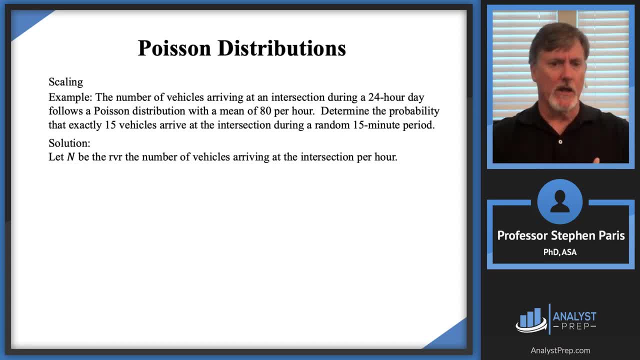 That's what I was given in that first sentence. I'm told that that's a Poisson distribution And I'm expecting to see 80 vehicles arrive per hour. So this cap n is a Poisson distribution with a parameter of 80.. 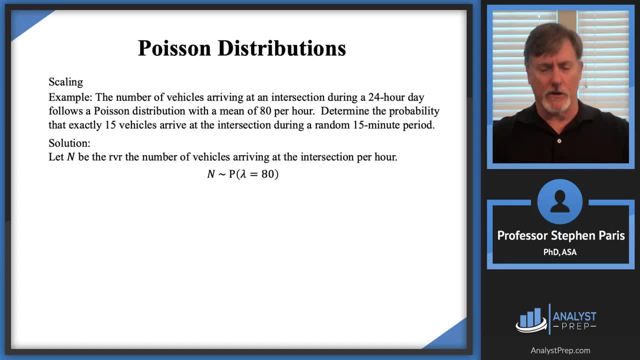 And now let's define another distribution or another random variable, cap n, tilde to be the random variable representing the number of vehicles arriving at the intersection during a 15-minute period. So the fact is that when I'm scaling here, I'm going to get another Poisson distribution. 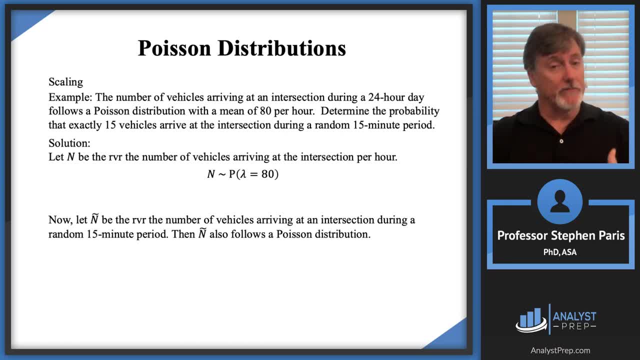 So cap n tilde is going to be a Poisson distribution. The question becomes: well, what's its parameter? What parameter do I use for it? And the parameter you can always get by. what do you expect to happen? So I'm expecting 80 vehicles to arrive. 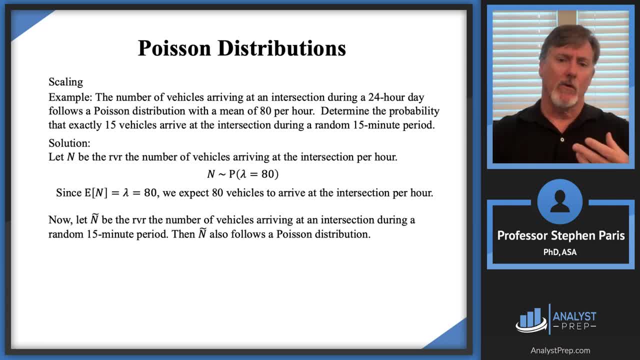 at the intersection per hour And in the scaling idea I'm scaling the per hour or the exposure unit hour to 15 minutes, And since 15 minutes is a quarter of an hour, then I'm going to expect one quarter of the 80 vehicles. 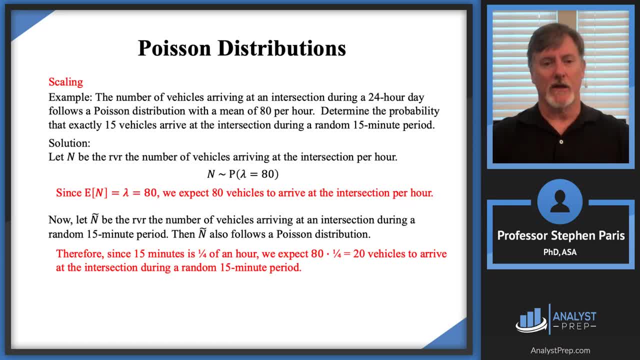 or 20 vehicles to arrive at the intersection during a random 15-minute period. That's just the property for Poisson distributions. That's a very nice property that takes place when we have Poisson distributions, And so we've scaled And the parameter then from an 80 to a 20.. 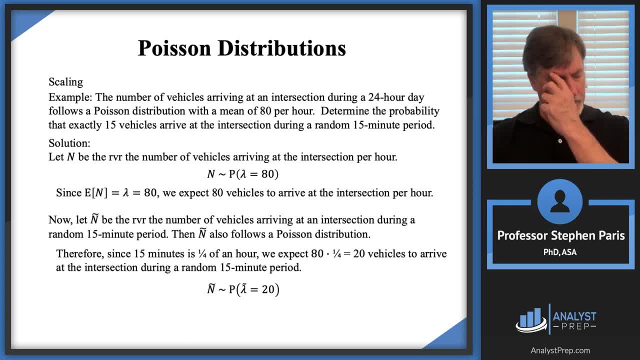 So if I'm counting the number of vehicles that arrive in a 15-minute time period, then I'm expecting 20.. So I'll use a parameter for 20 for the cap n tilde random variable And I'll call that parameter lambda tilde. 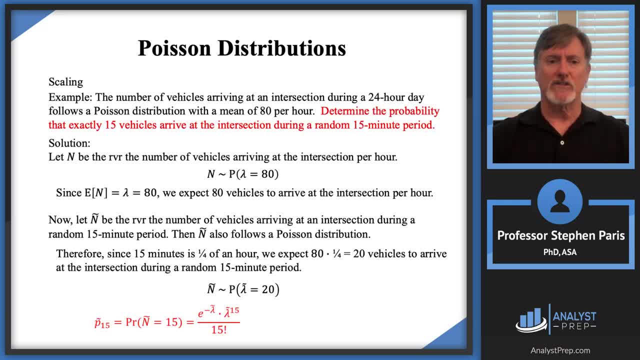 And then the question is: well, what's the probability that exactly 15 vehicles arrive during a 15-minute period? So the number that arrived during a 15-minute period is a Poisson distribution, And that's a Poisson distribution with a parameter 20.. 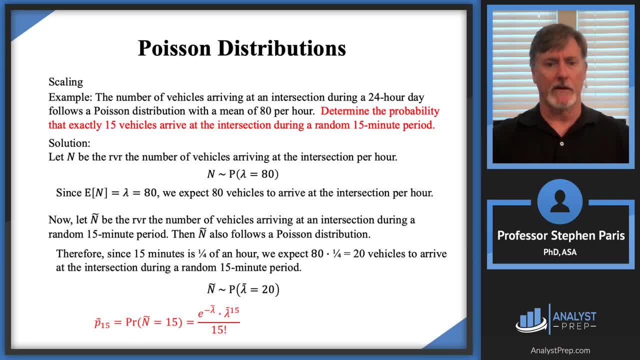 So the probability that I get 15 vehicles arriving during that time period would be e to the minus lambda, lambda to the 15 divided by 15. factorial. using a 20 now as the parameter, Do the arithmetic here And I got a little bit more than 5% when I did the calculation. 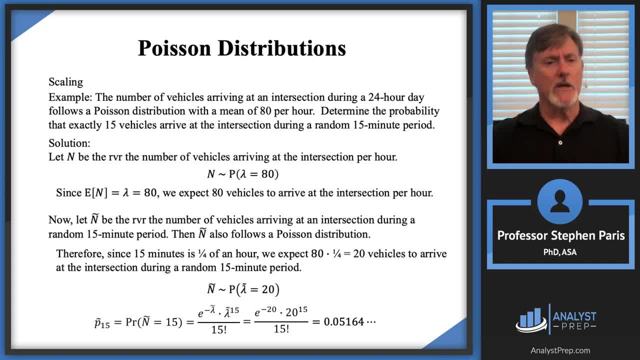 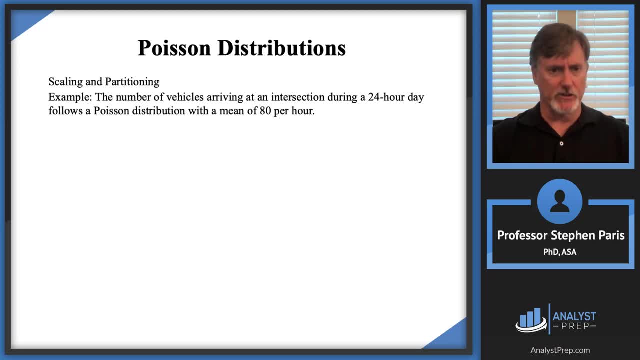 I got a little bit more than 5% for that probability. So I mentioned before we were going to talk about scaling and partitioning. So that was an example of scaling And I'm going to go back to the exposure unit. Now let's look at an example of partitioning. 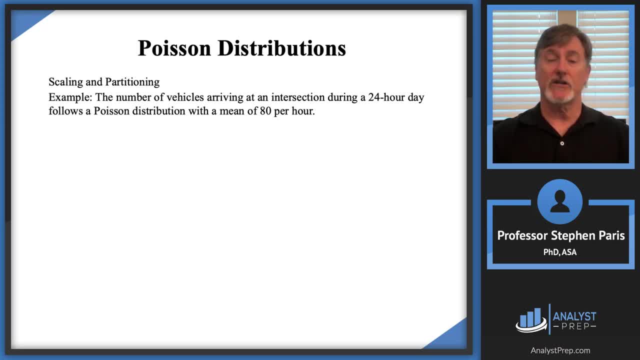 We're going to start with the same setup: that we have vehicles arriving at an intersection And we're expecting 80 vehicles to arrive per hour. But now let's partition the vehicles into trucks. Let's say 10% are trucks, 25% are SUVs and the rest are cars. 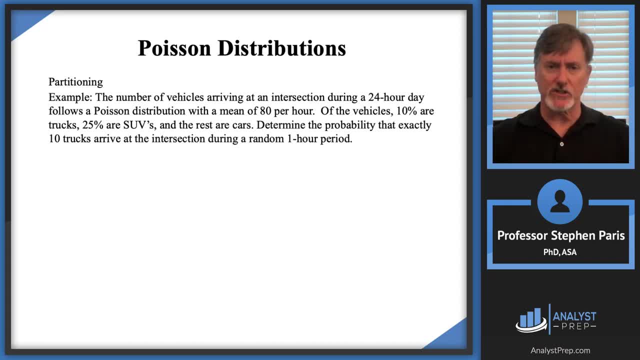 And so I've partitioned the vehicles, The objects that we're counting. I've partitioned them now. So this is an example of partitioning. The point is that there's a very large probability that exactly 10 trucks arrive at the intersection. 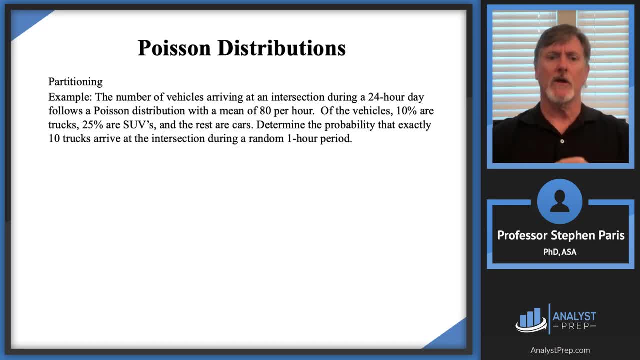 during a random one hour period. So with the exposure unit, I'm not doing anything with the exposure unit here. The first line here is that the number of vehicles arriving or arriving per hour, And then the question is the number of trucks arriving per hour. 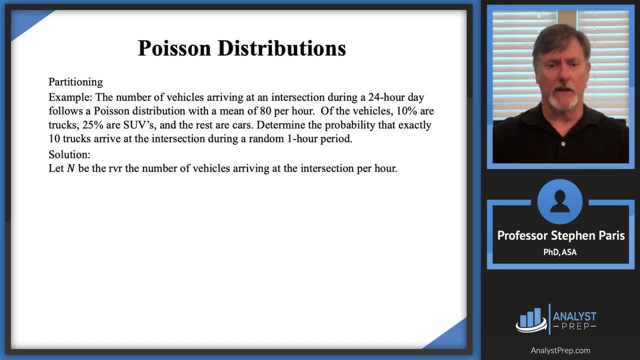 So I haven't done anything with the exposure unit. I've only partitioned the objects that we're counting, So we'll cap in being the random variable representing the number of vehicles arriving per hour. I'm expecting 80 vehicles to arrive per hour, so it's a Poisson distribution with parameter 80.. 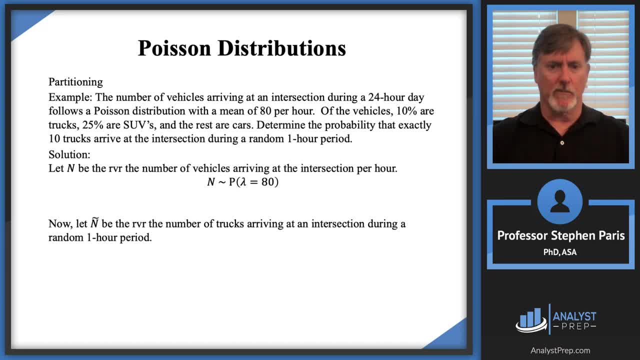 I'm going to define this new random variable, cap N tilde, to be the number of trucks arriving at the intersection during a one-hour, random, one-hour period. So the fact, with Poisson distributions, when you partition you're also going to get another Poisson distribution. 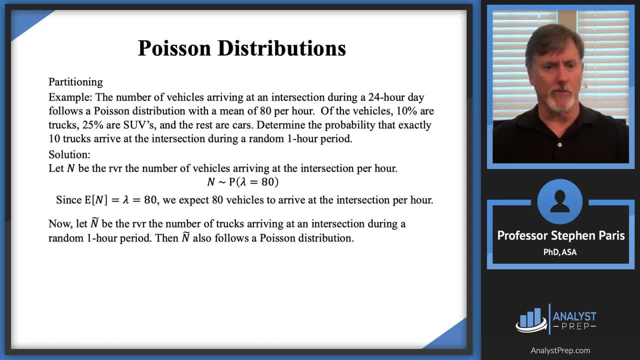 That's nice. So what's the parameter? Well, the original parameter being 80 means I'm expecting 80 vehicles to arrive at the intersection per hour. 10% of the vehicles are trucks, so I'm going to expect 10% of the 80 or 8 trucks to arrive at the intersection. 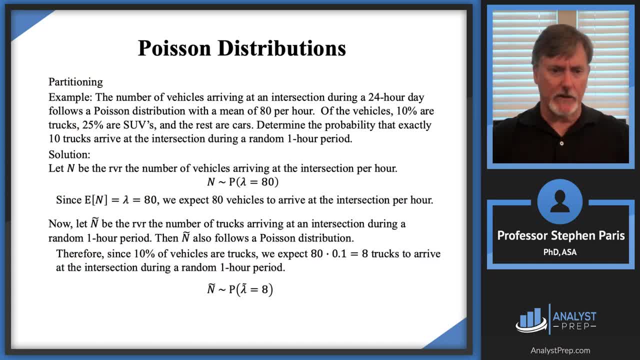 during a random one-hour period, And so my cap N tilde random variable is going to be Poisson with a parameter of 8.. I'm expecting 8 trucks again to arrive. Cap N tilde is counting the number of trucks per hour and I'm expecting 8 of them, so that's my parameter. 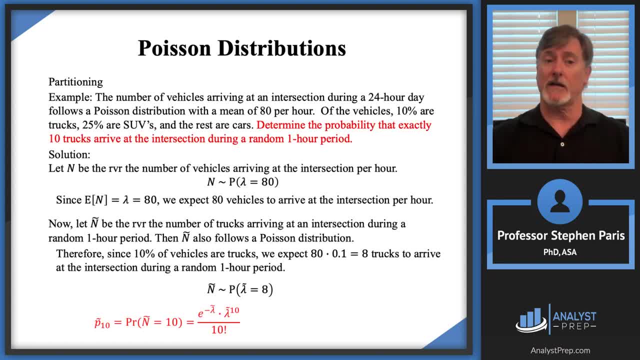 And then the question, though, is: well, what's the Poisson distribution? What's the probability that exactly 10 do arrive at the intersection? So that's the e to the minus lambda, lambda to the k divided by k factorial. 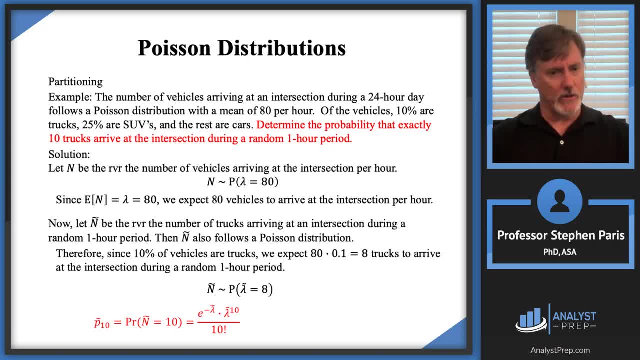 I'm plugging in a 10 for k and this time, if I'm counting trucks, I'm going to use the parameter 8 for lambda and I get this e to the minus 8 times 8 to the 10th divided by 10. factorial. 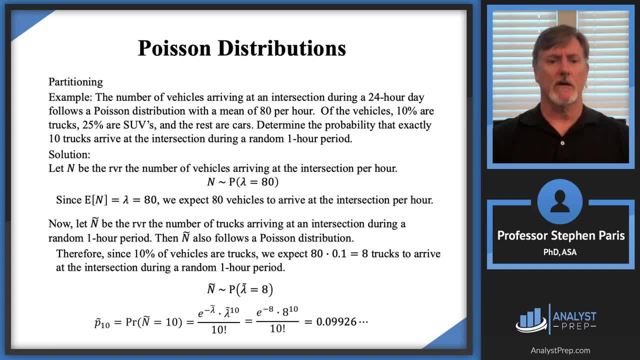 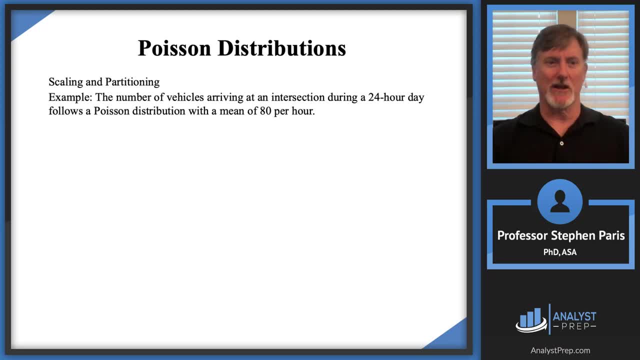 And when I did that calculation I got just under 10% when I did the calculation there. So again, we talked about scaling and partitioning. We did this example with scaling, We did the example with partitioning. so you probably know what's next. 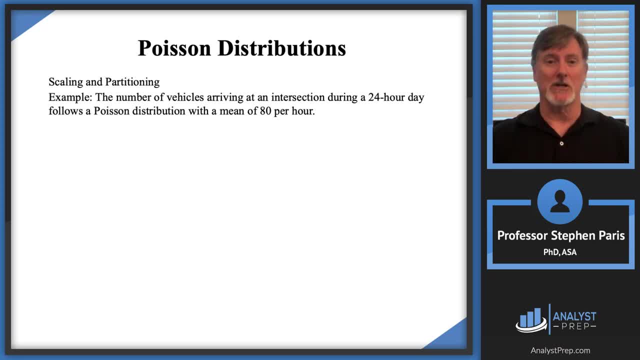 We're going to do both scaling and you can both scale and partition. So let's, same setup We got. we're expecting 80 vehicles to arrive at this intersection per hour- 10%, let's. we're going to assume 10% of the vehicles are trucks. 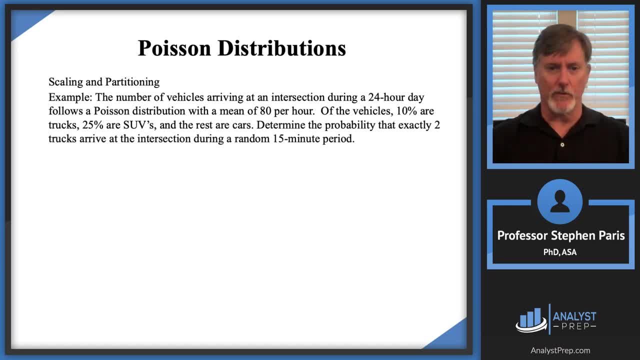 25% are SUVs and the rest are cars- at any time on the road. And the question now is: what's the probability that exactly two trucks arrive at the intersection during the random, A random- 15 minute period? So I'm partitioning the objects that I'm counting into trucks, SUVs and cars. 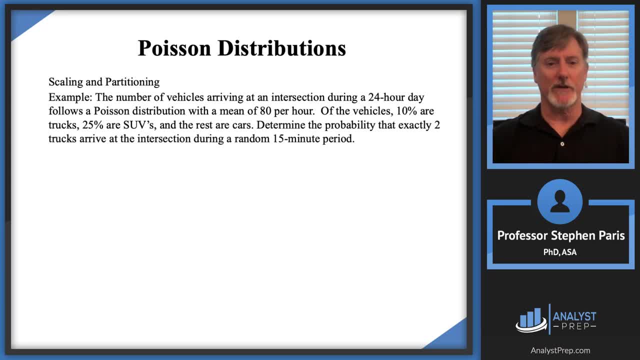 and I'm scaling the exposure unit from an hour to a 15 minute period. So I'm going to set it up the same way with cap in being the random variable that's following this Poisson distribution, with with parameter 80. It's the number of vehicles arriving at the intersection per hour. 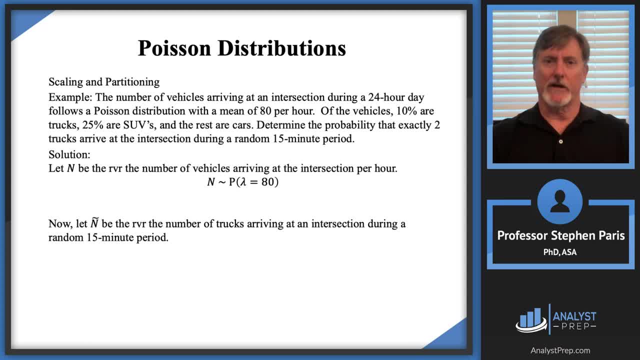 Cap in tilde I'm going to be. I'm going to define as the random variable representing the number of trucks arriving at the intersection in a 15 minute period. The fact is that it will be a Poisson distribution, since I'm expecting 80 vehicles to arrive. 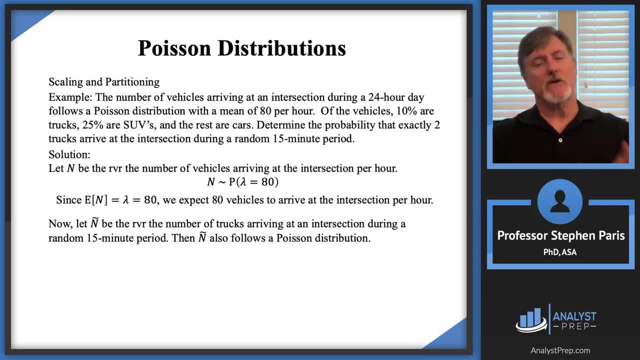 at the intersection per hour and of the 80, 80 vehicles to arrive per hour. I've got now I'm counting over a 15 minute period, So 15 minutes is is a quarter of an hour or 0.25 of an hours. 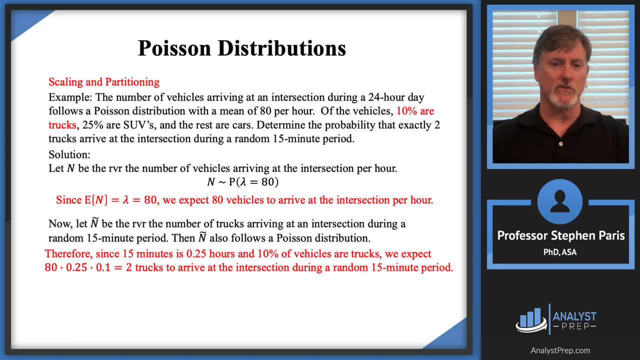 I'm not counting vehicles anymore, I'm counting trucks, and 10% of the vehicles are trucks. So over that 15 minute period I'm going to expect, of the 80 that we're arriving during the hour, a quarter of them are going to arrive at the intersection. 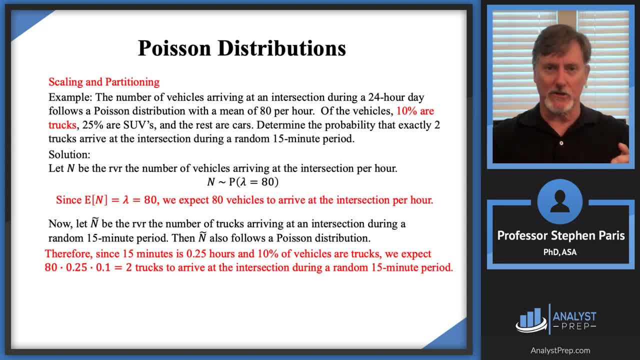 I'm going to expect the truck to arrive during the 15 minute period. So now it's 20, down to 20 vehicles arriving over a 15 minute period, and of those, 10% are trucks. So 10% of the 20 is 2..